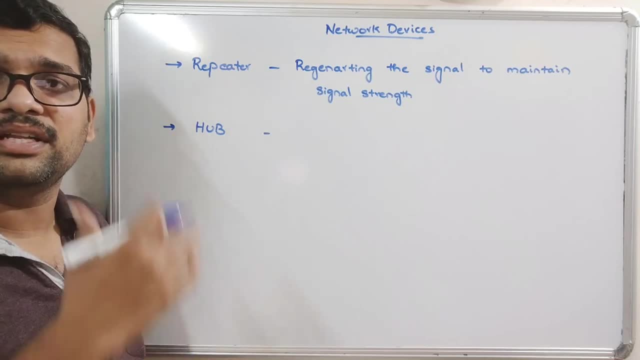 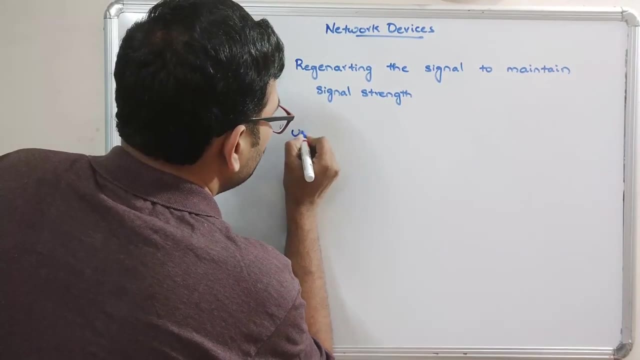 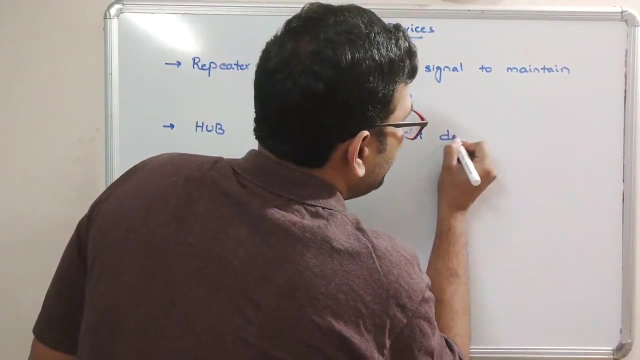 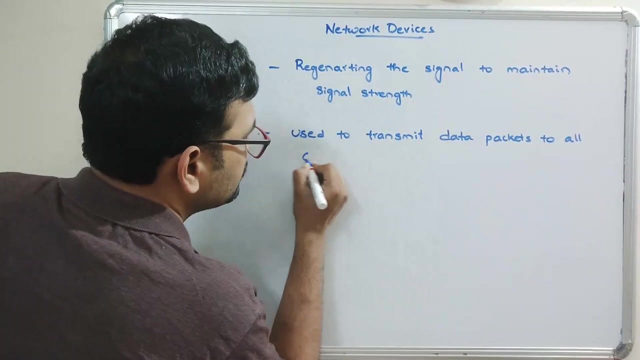 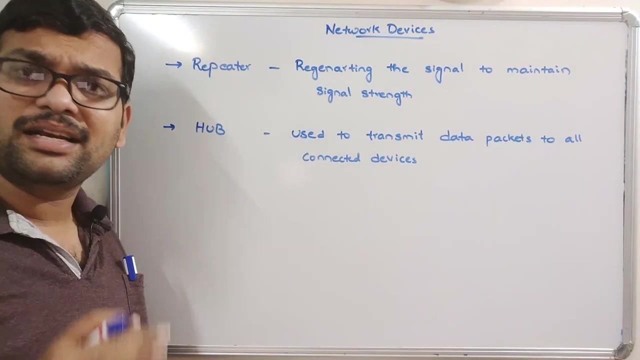 unit that is called hub, And whatever the data received in this hub, that will transfer the packets to all the connected devices. Okay, so use it to transmit data packets to all connected devices. So it doesn't have any filtering option, So it doesn't verify anything, just it will send the. 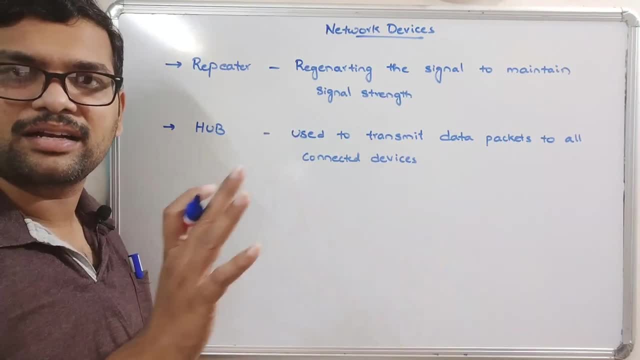 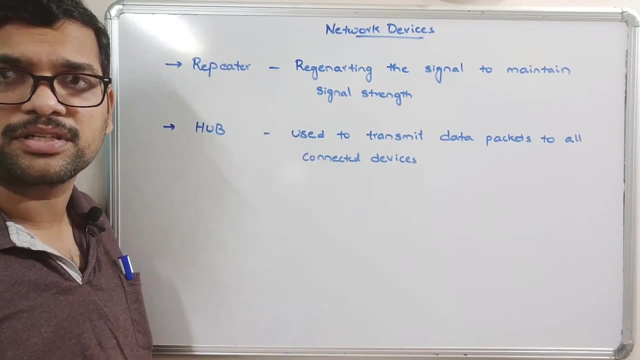 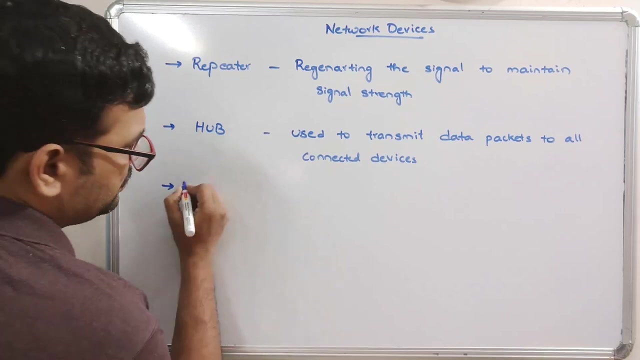 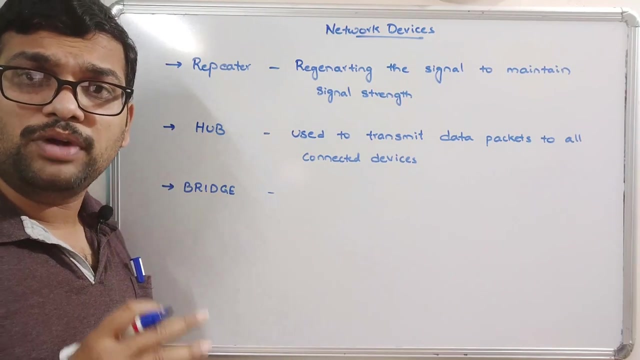 data packets which have been received by this hub to all the connected devices. right, There is no routing, there is no path or there is no any other filtering options here. right? So this is hub And the next one is bridge. This bridge is mainly used to interconnect two different 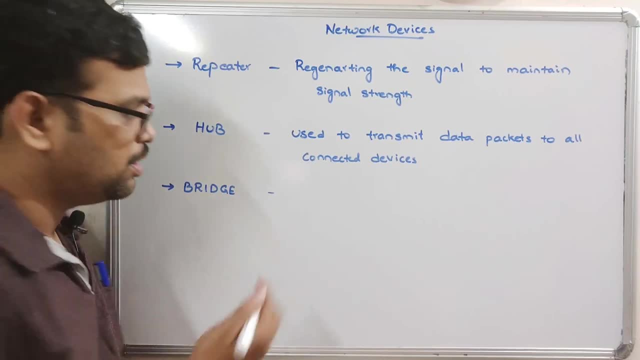 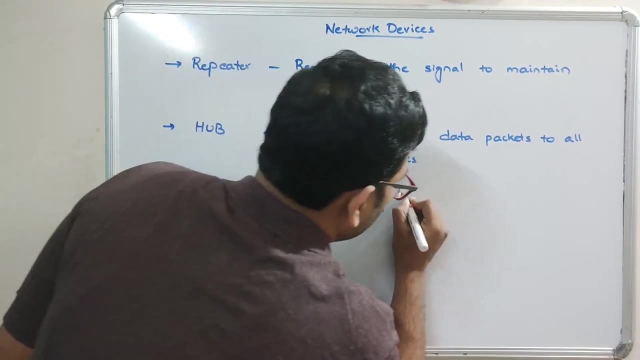 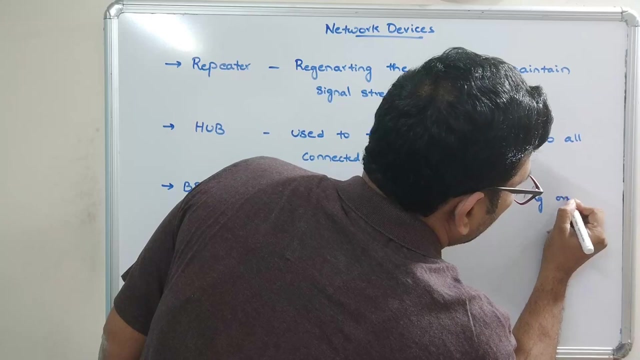 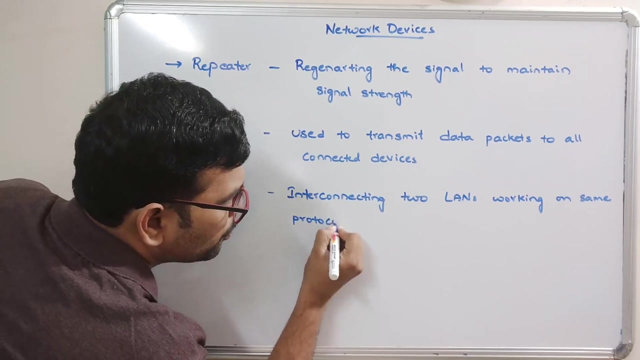 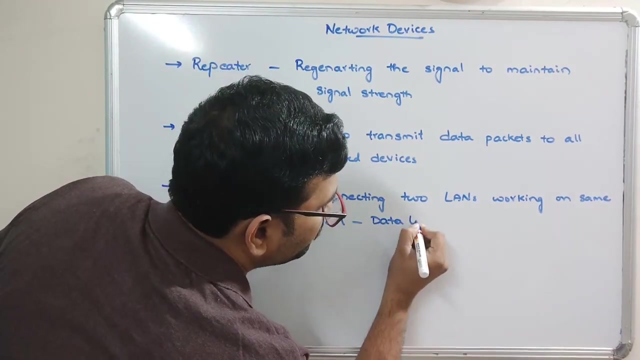 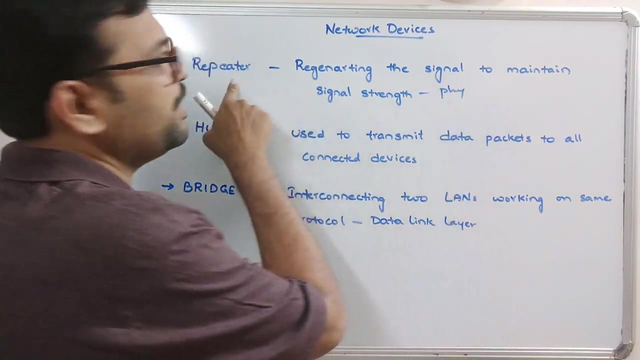 LANs in the same protocol working on a same protocol. So interconnecting two LANs working on working on same protocol. okay, same protocol and this will be used in data link layer, data link layer and this is in physical layer. this repeater will be operated in physical layer. 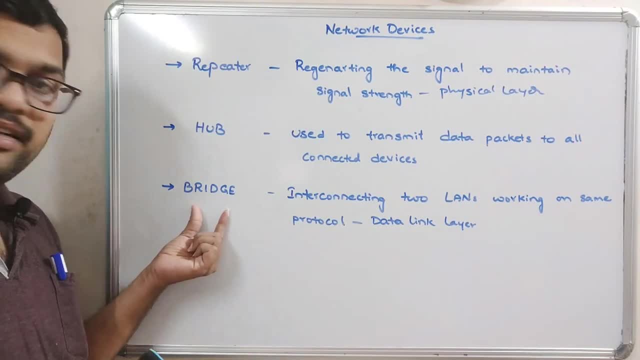 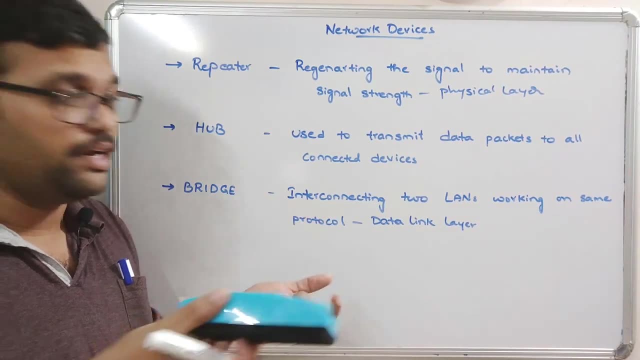 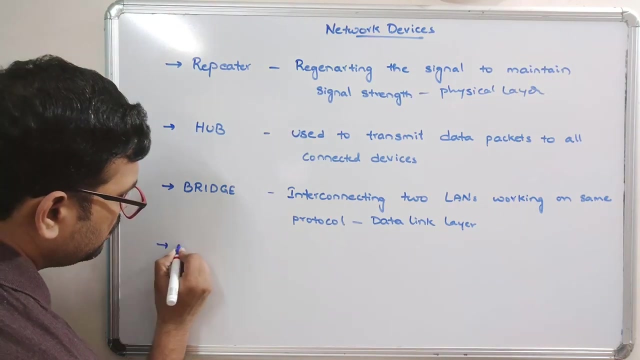 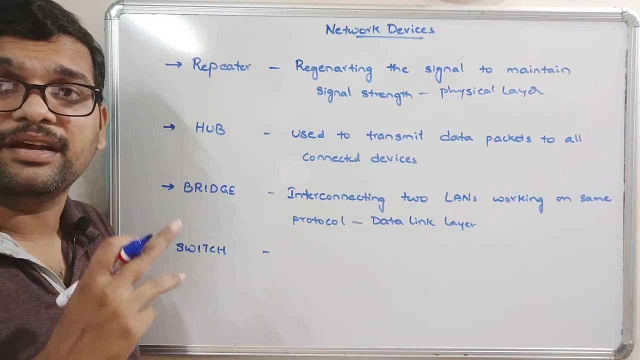 right, Right, so a bridge- the name itself indicates so that will be acting as an interfere, I mean intermediate between two different networks which are operated in the same protocol, on same protocol, so working on same protocol, and the next one switch. so switch is similar to our repeater with some additional functionality. so what is? 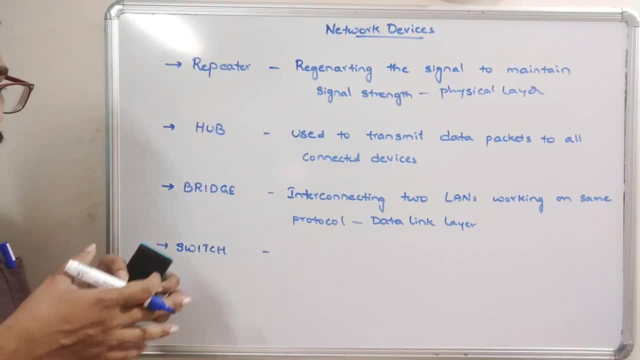 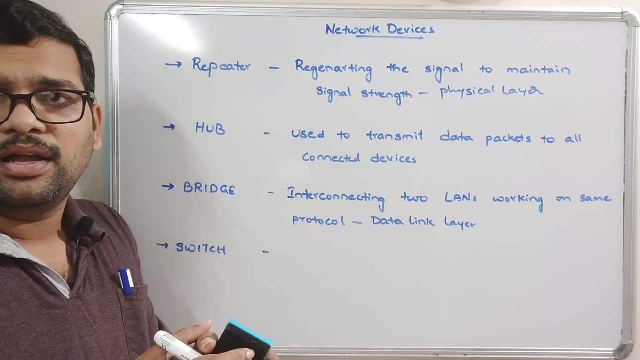 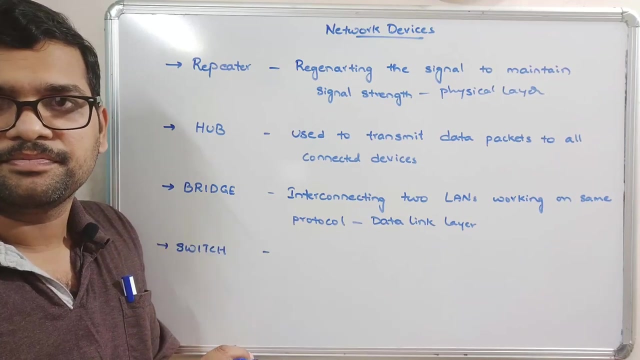 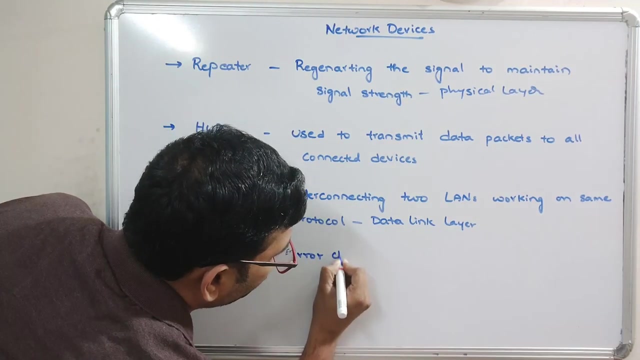 that additional functionality. so switch will send only the correct and good data packets to the ports and whatever the error. if the packets contain some error, automatically those packets will be ignored by the switch. so error checking will be done here. okay, switching in switch, so error checking will be done. 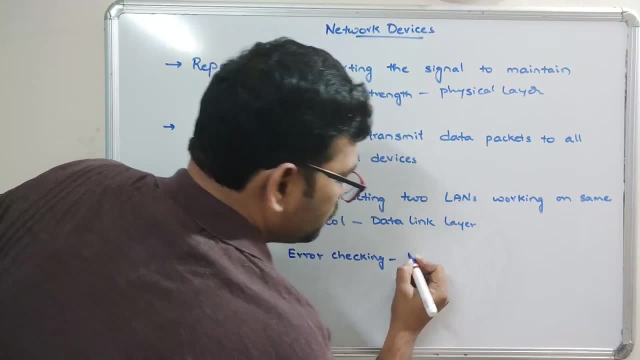 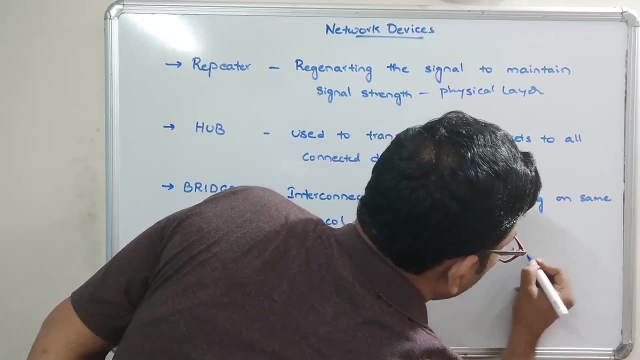 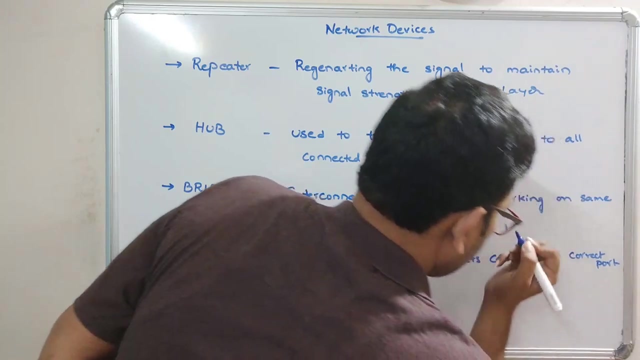 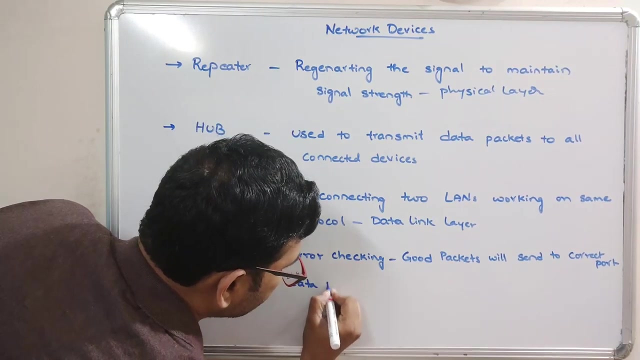 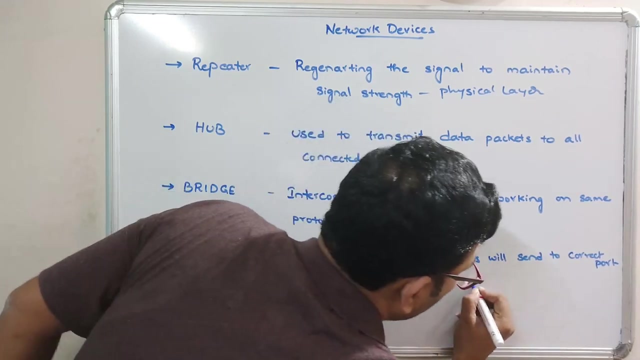 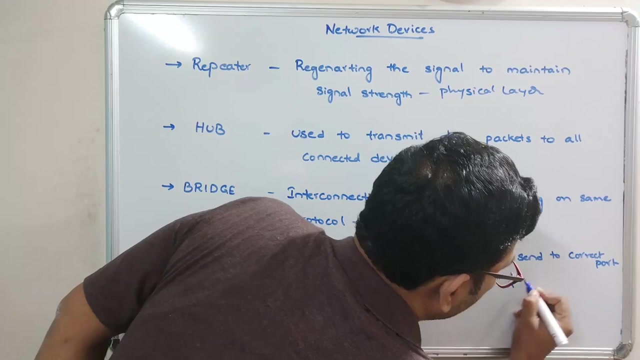 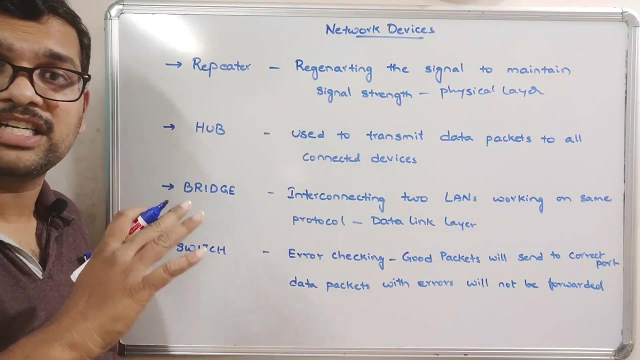 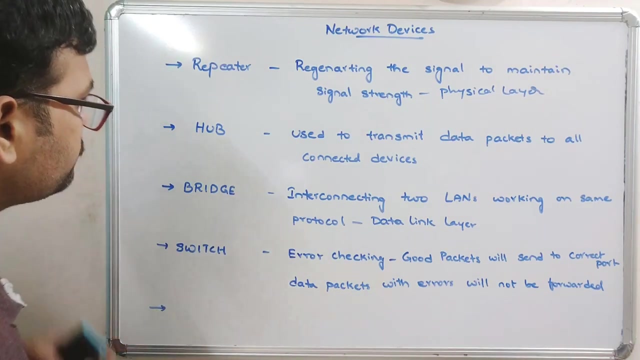 error checking. so what kind of error checking? so Good data packets, good data packets can send to correct port, right, and data packets, data packets with errors, will not be forwarded. will not be forwarded, So those packets will be ignored. will not be forwarded, right, So those packets will be ignored there itself. and the next one: 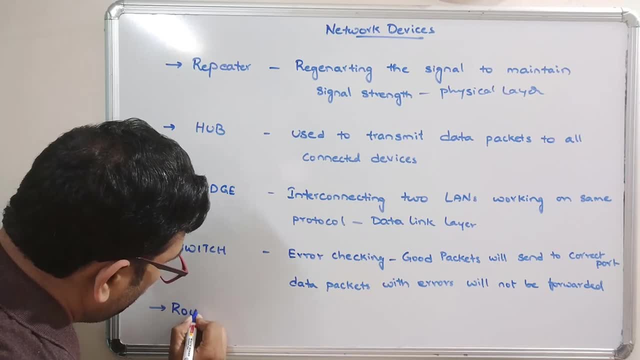 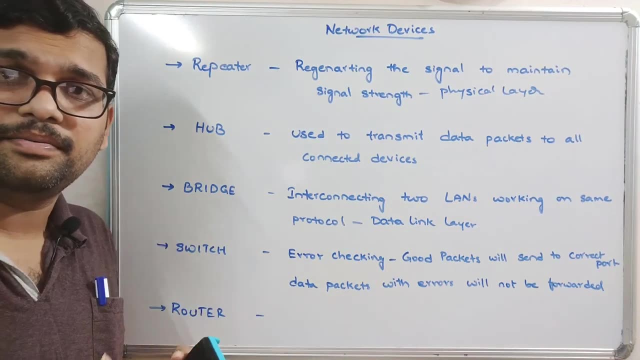 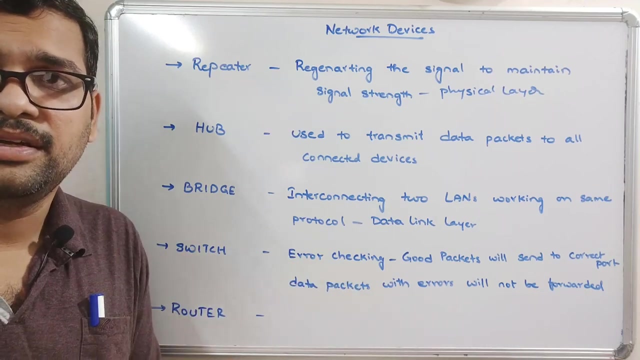 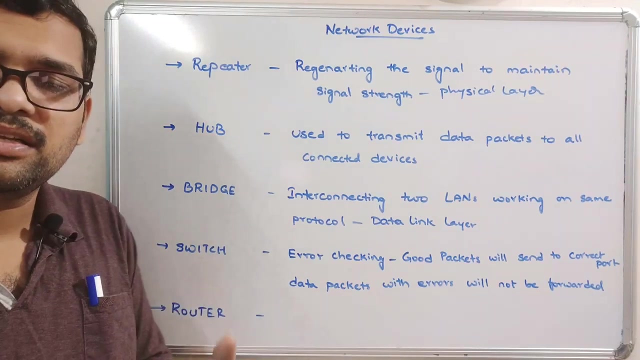 router. So router will collect the data and it will send to the different ports based upon the IP address. So, based upon the IP address, the data will be send to the destination right by using the different routing algorithms. So all the routing algorithms will be here. 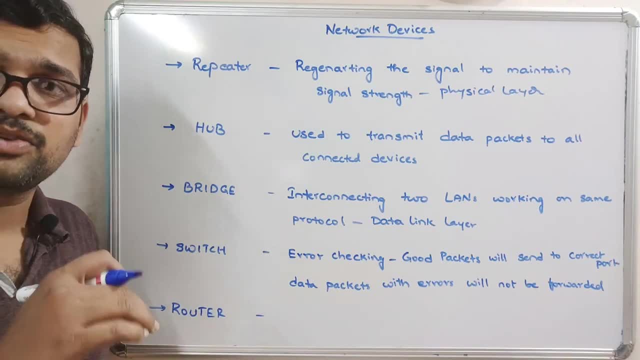 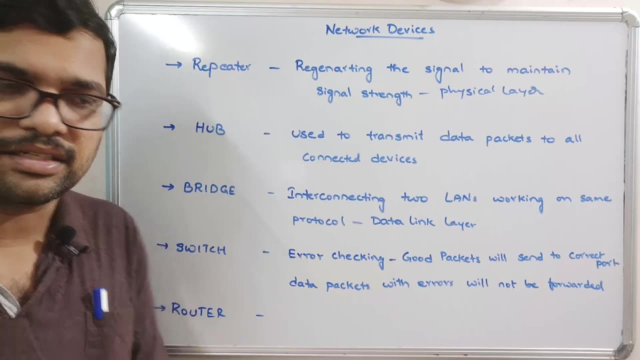 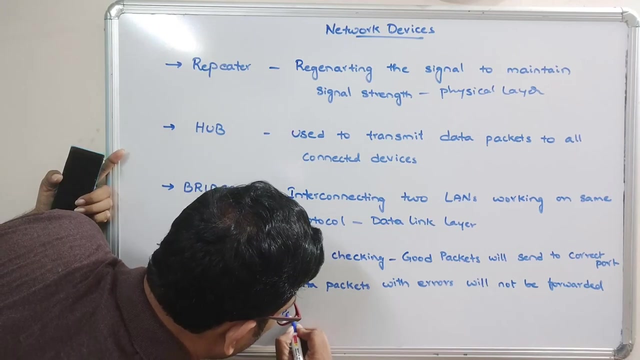 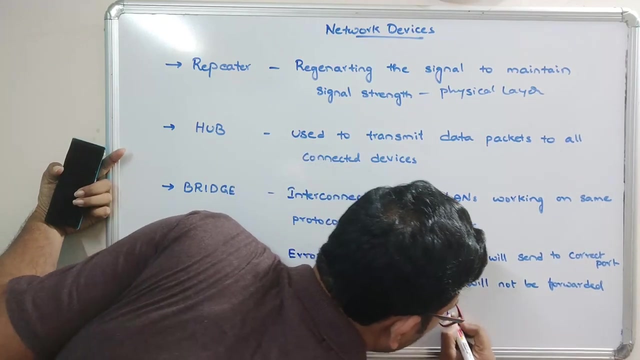 and the routing will be done here. here and the best routing path. it will select the best routing path and through that routing path the data packets will be sent to the destination. so that will be done by the router. okay, so packets will be rooted to destinations. 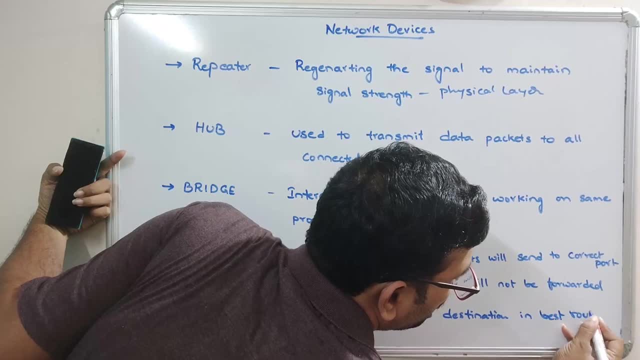 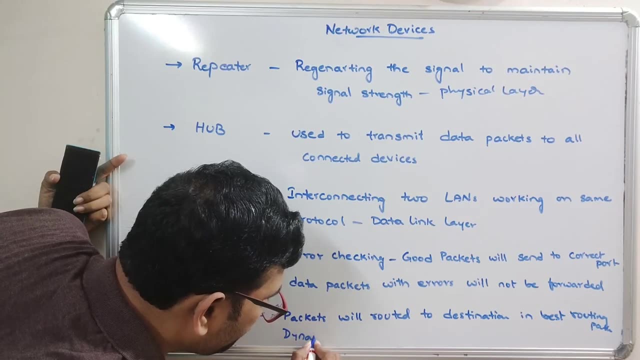 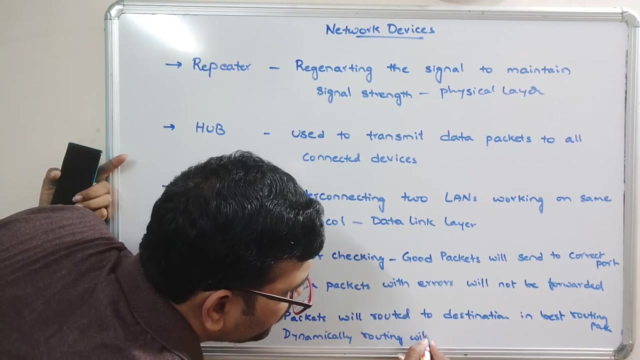 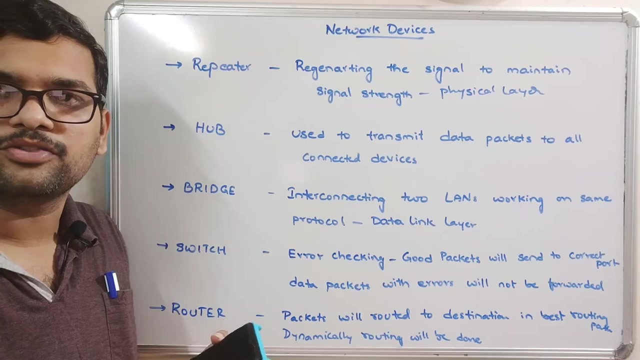 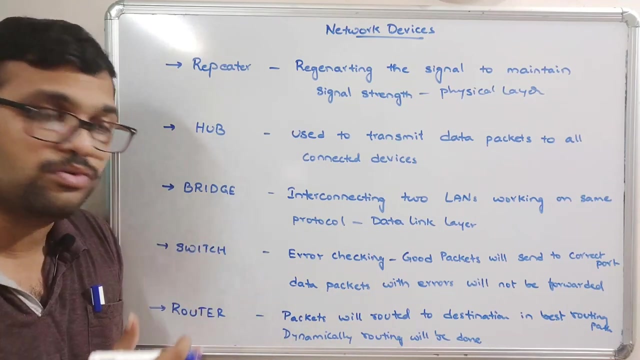 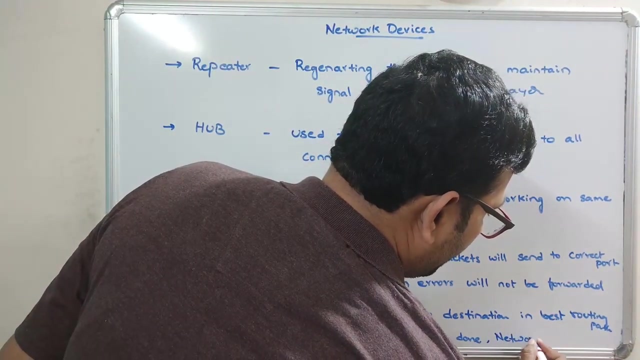 in best routing path and here, dynamically, routing will be decided. okay, dynamically, the routing will be changed from one packet to another packet, so it will select the best path and through the best path the routing will be done in this router and this will be operated in network layer. network layer. this will be operated, operated in network layer. 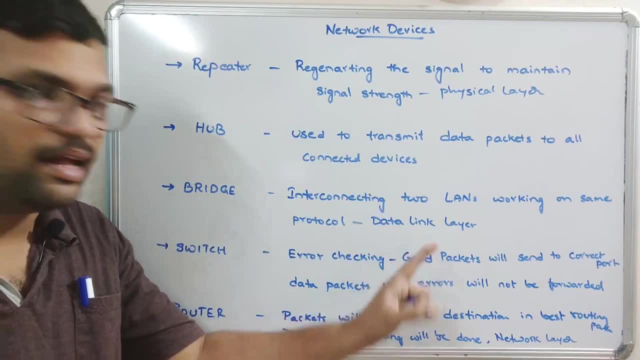 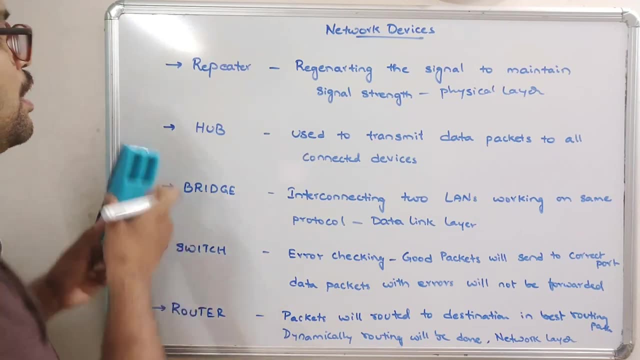 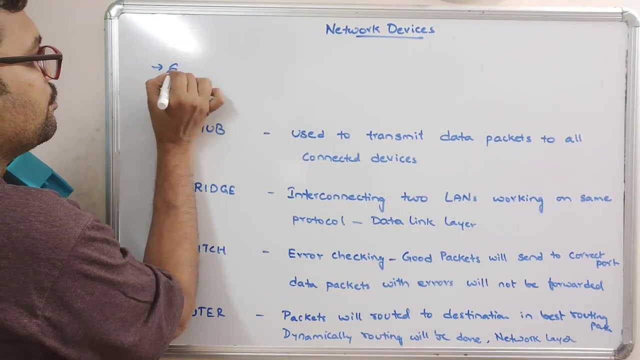 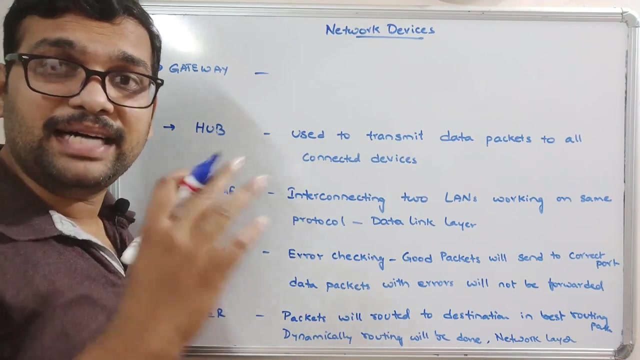 right, so this will be in the physical layer, this will be in the data link layer and this will be in the network layer, right so? repeater, hub, bridge, switch and router. now the next one is gateway- gateway, so the name itself indicate gateway. it passes the data from one, I mean from one. 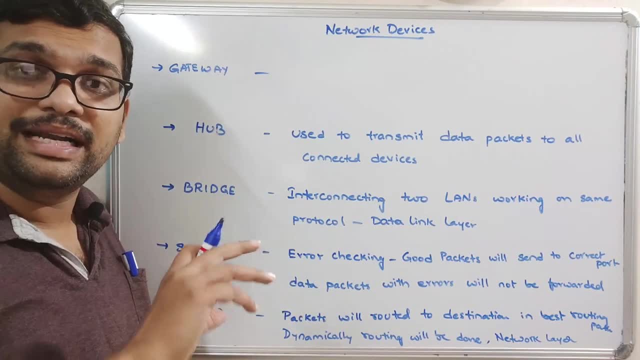 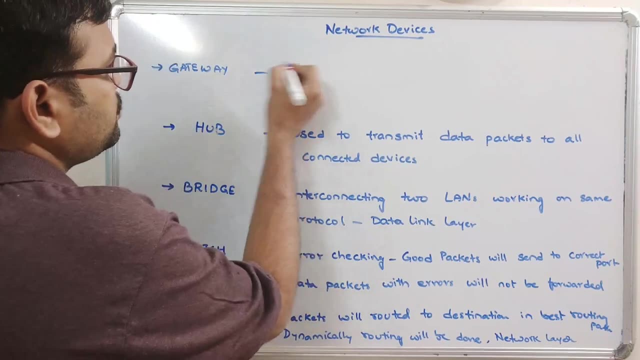 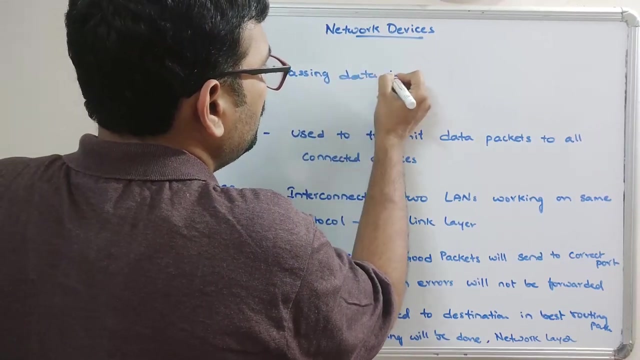 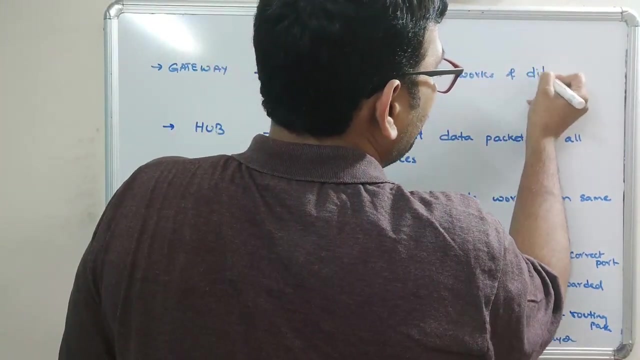 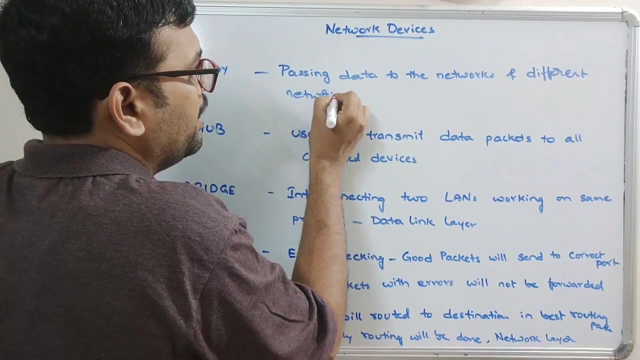 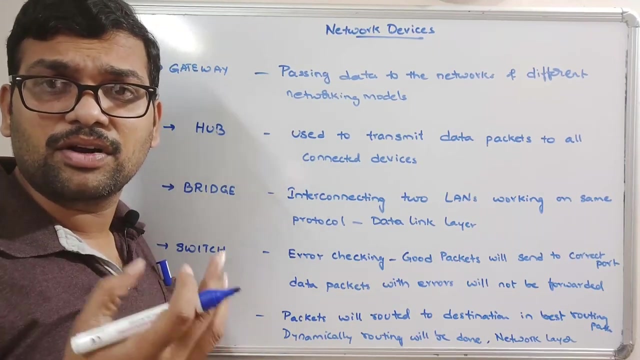 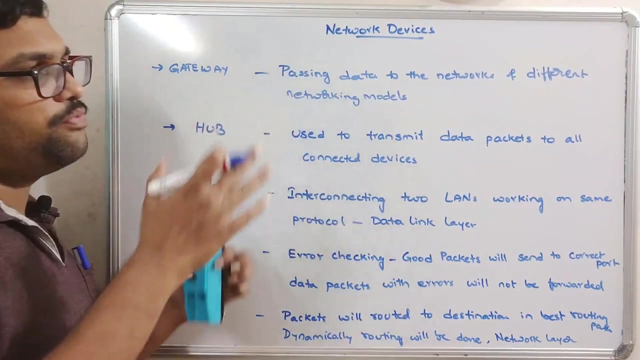 network to another network which are handling in different protocols, which are using the different protocols or a different network models. right, so here passing data to the networks of different networking models. so we are having different networking models, just like our OSI model and TCP model. right, so here the passing of data that. 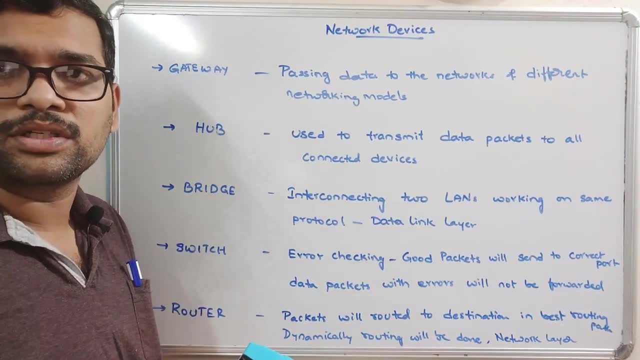 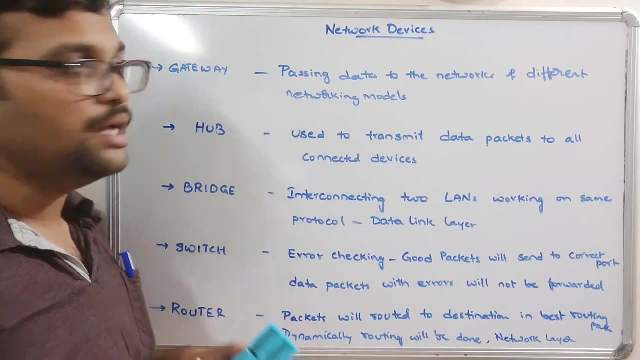 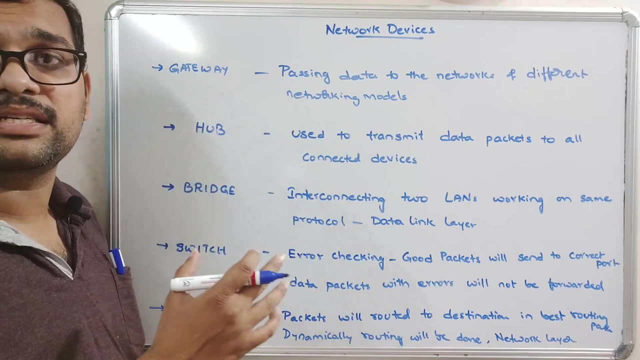 means the interconnection between two different models, network models. so first we will get the data and that will be interpreted and that will be sent to the destination right. so that is the usage of this gateway. so these are the basic network devices we will use in the networking. so repeaters, hub, bridge. 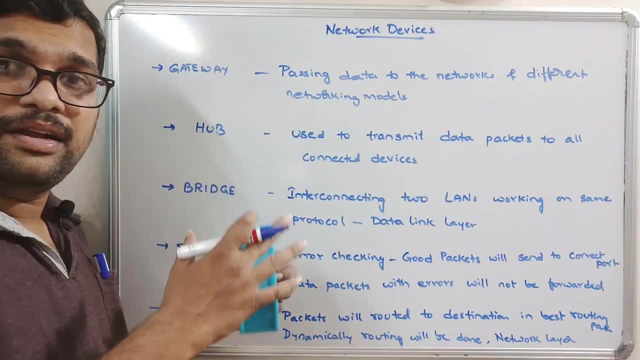 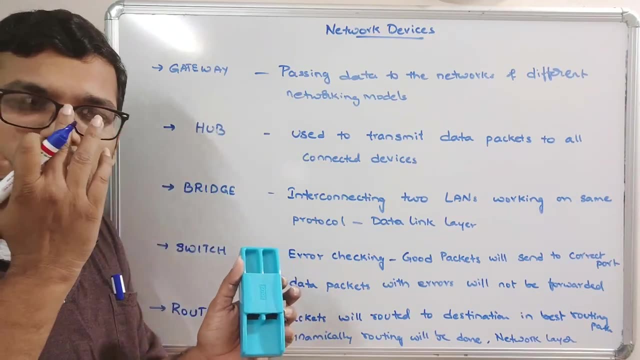 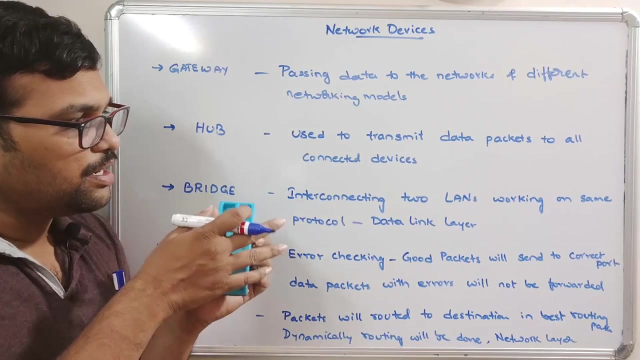 switch and router right. so repeater is simply: it will regenerate the signal and hub will simply transmit the data packets to all the ports or all the connected devices and, coming to the bridge, based upon the MAC address, so it will connect. I mean the data will be processed and it is nothing but an. 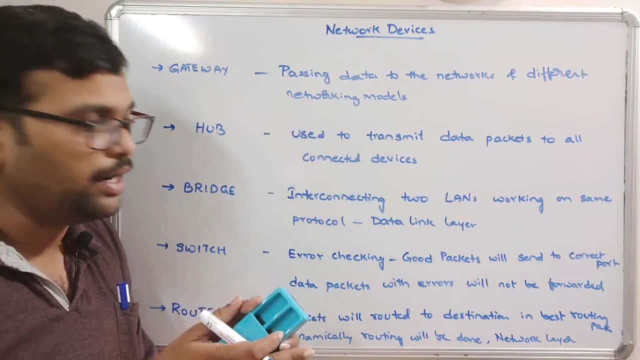 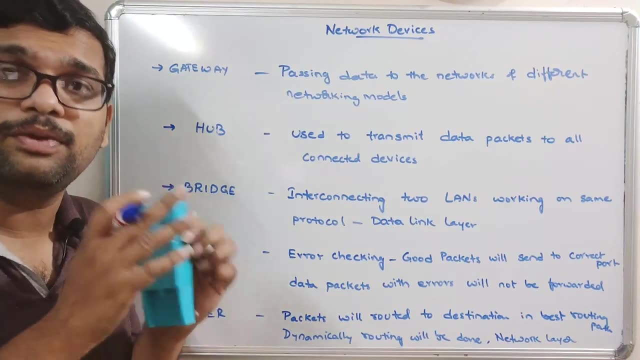 interconnection between two different LANs working in the same protocol. right, and coming to the switch. here the error checking will be done and whatever the packets which are having the errors will be ignored here itself and only the good data packet. that means without any error the data packets will be.